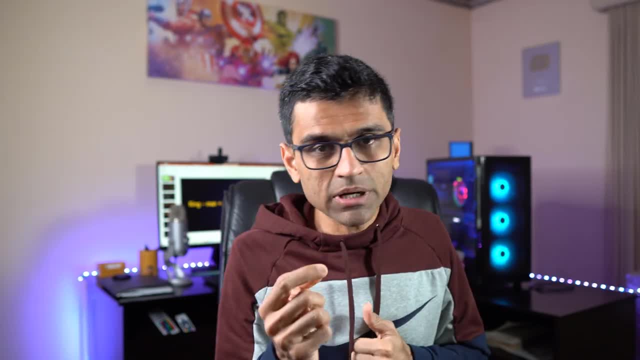 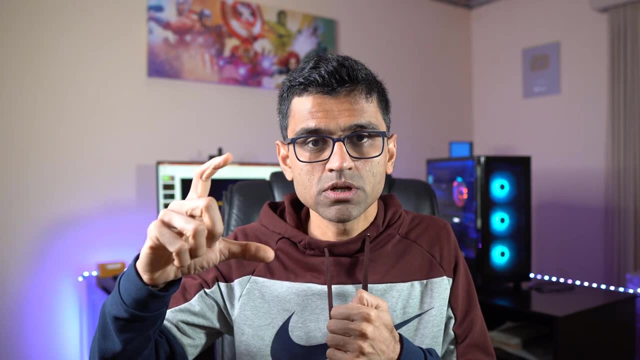 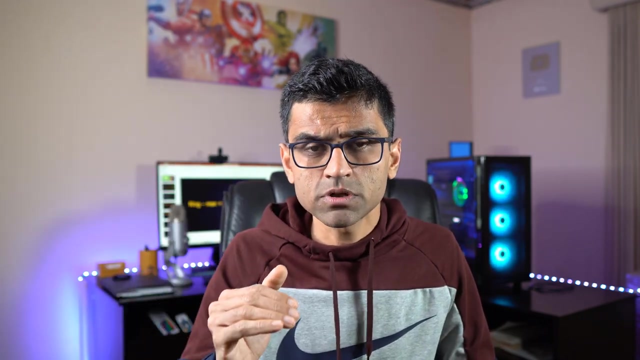 represent the meaning of the word king. Now that number cannot be one number, so you need to have set of numbers, and in mathematics set of numbers are called vectors. So let's think about this: How about we represent word king into a vector, which is just a bunch of numbers, such that it can represent the meaning of word? 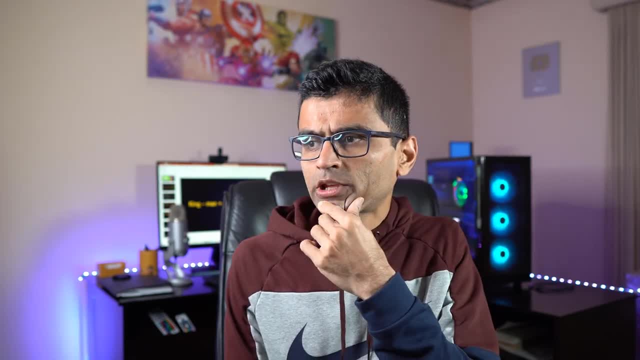 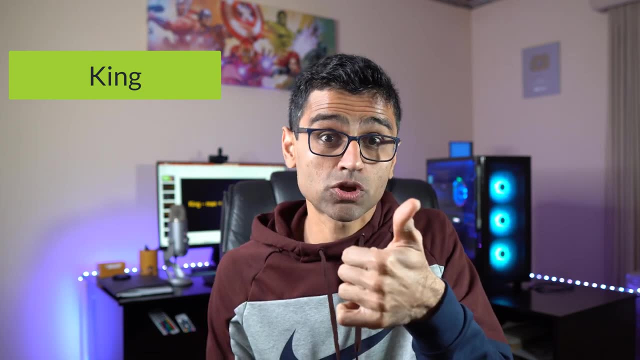 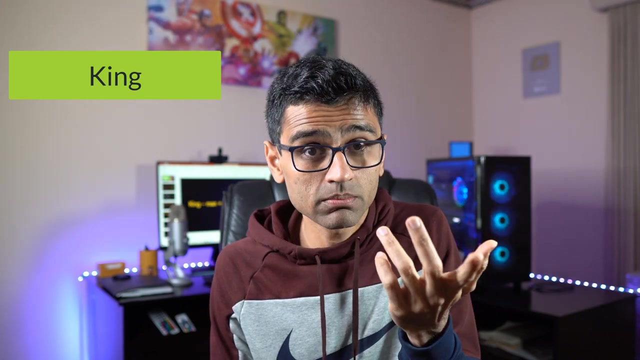 king accurately. Now think about king. King has a different property or there are different ways of representing the word king, For example, king has authority, King is rich. usually King has a gender of male. okay, Does king have a tail? No, generally horse. 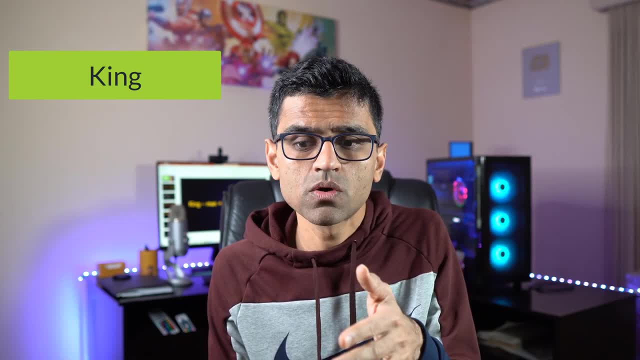 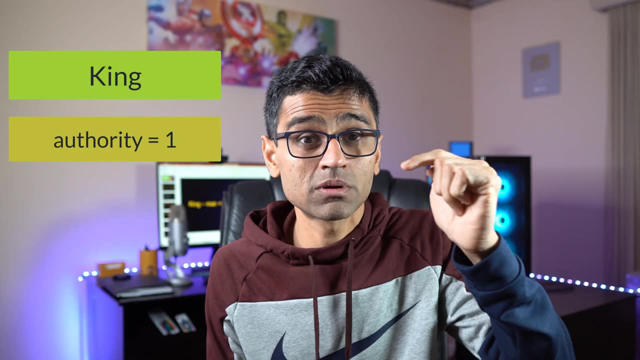 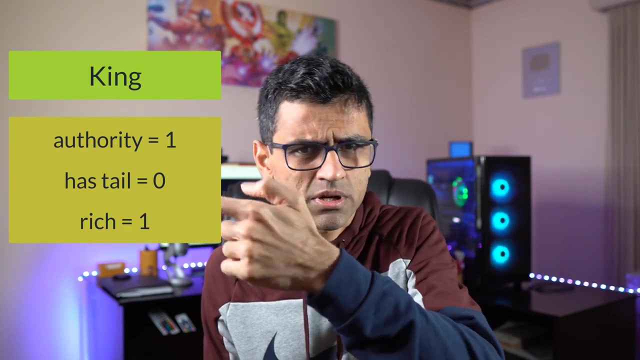 will have a tail, right? so that answer will be zero. so what if we do this? all right. so for authority, we'll give number one. for tail, we'll give number zero, because king doesn't have tail. for being rich, we'll give number one: one meaning super rich, zero meaning very poor. and for gender: 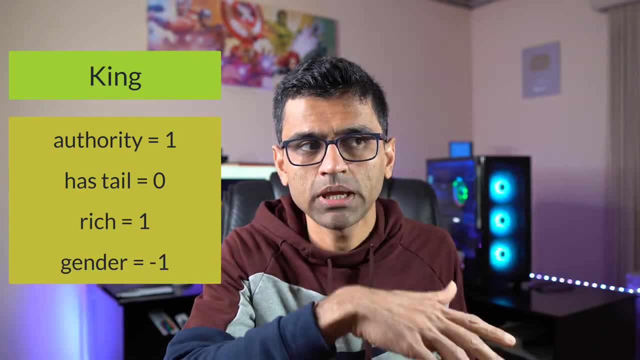 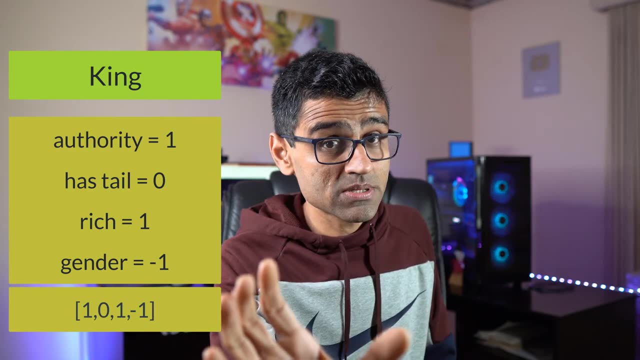 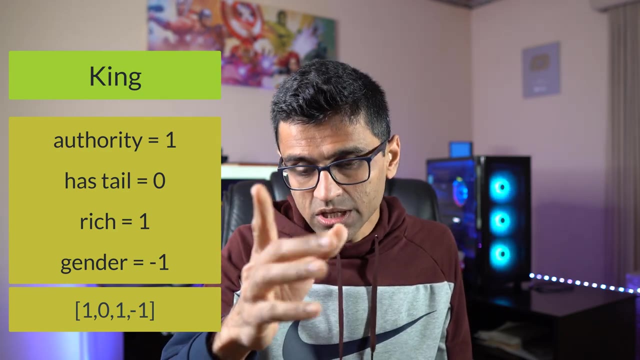 let's say we give number minus one. minus one is male and one is female. now we came up with this vector: 1 0, 1 minus 1. that represents the meaning of word king. you can do similar thing with another word, for example horse. for horse, the property tail will be one, but the other properties, such 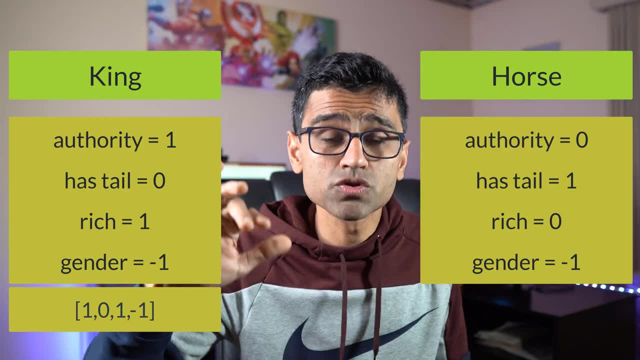 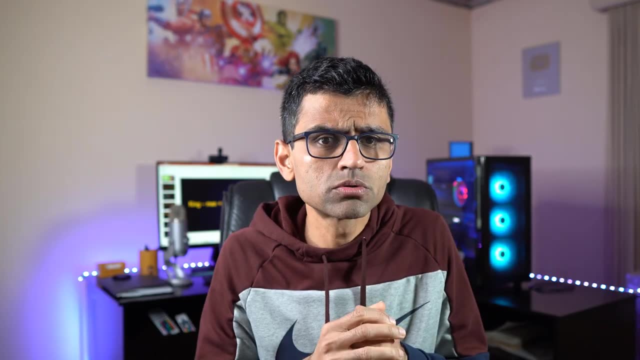 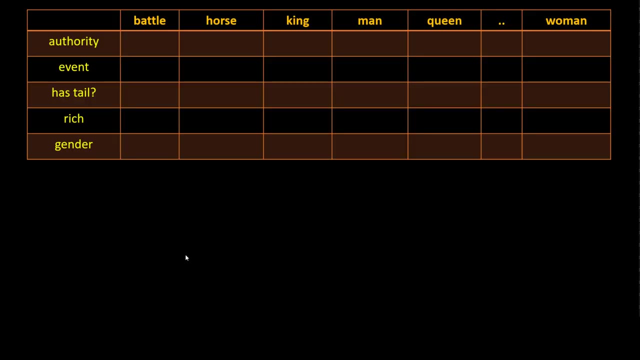 as authority, being rich, etc. will be close to zero. and if you do this for all type of different words in your vocabulary, you will be able to do a math. so let me just show you a very simple example here. you let's say i have a story of king and queen and i want to represent all the words in that story with 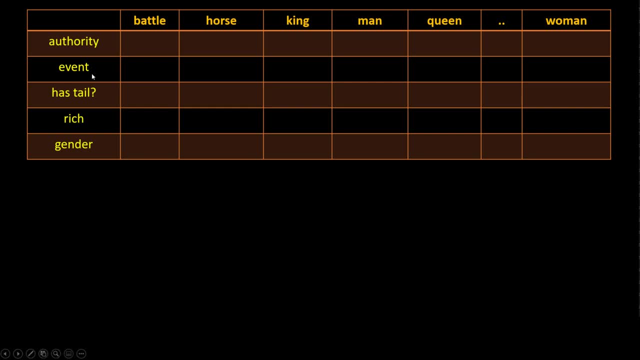 word vectors. here i have different properties, such as authority, event has tail and so on. and let's say there is a word called battle for battle, battle is an event, so the that value is one. remaining values are zero. horse has a tail, that's why it's one. horse might have little authority. 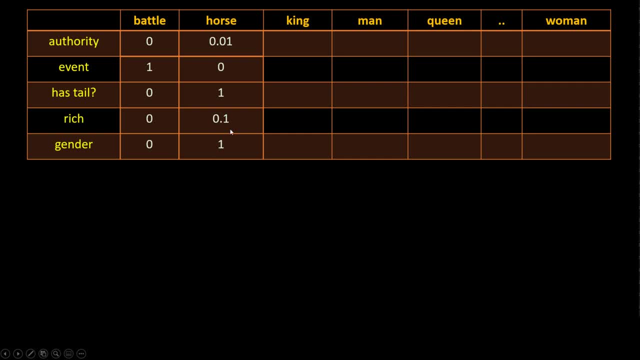 point zero: one horse might be a little rich. point one if it is a horse of a king. so, and gender is one here, like values, might not be zero, because i'll tell you the reason behind that a little later, but when you have king, we already saw, it's one zero. 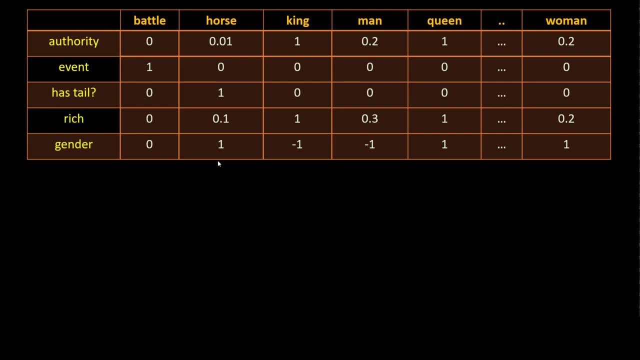 zero, one minus one. and for different words you can come up with these different type of vectors. and once you have the vectors you can do the mathematics. so now, when i do king minus men plus woman, you can do the mathematics. so now, when i do king minus men plus woman. 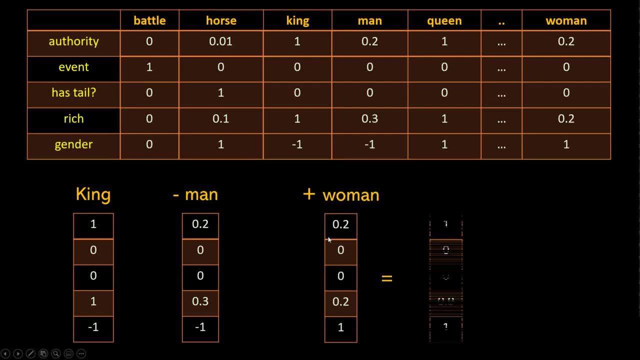 just do a simple math: one minus point two plus point two is one zero, zero. i'm taking individual elements. okay, one minus point three is point seven, plus point two, point nine, and that result vector is similar to a vector of queen. it is not exactly same, but it's quite similar. 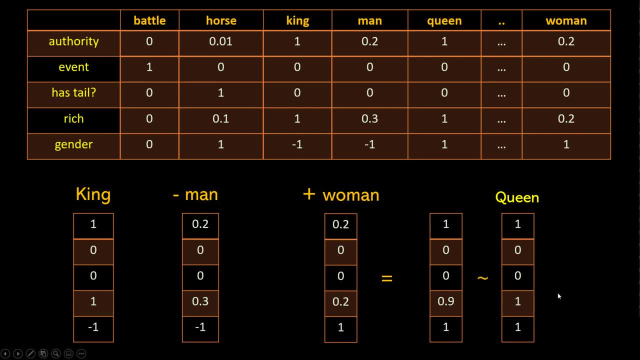 right point nine and one. that's the only difference. so you already saw how that math works. when you give this equation to computer, computer will be able to tell you that the answer is queen, and that is pretty powerful. now you don't want to hand code all these properties. 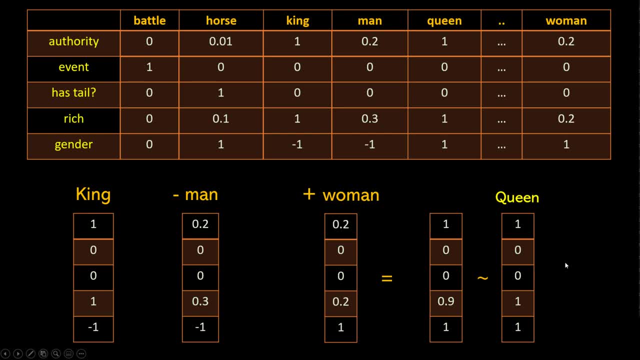 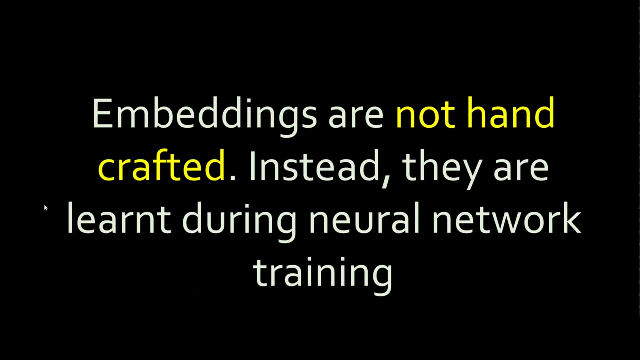 for all these words. let's say you're doing doing natural language processing for all the text on wikipedia. there are so many thousands of words and to come up with these kind of properties for each of these words will be very, very difficult, so you don't want to handcraft it. 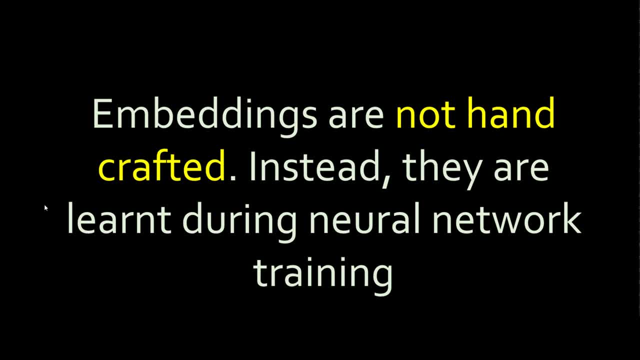 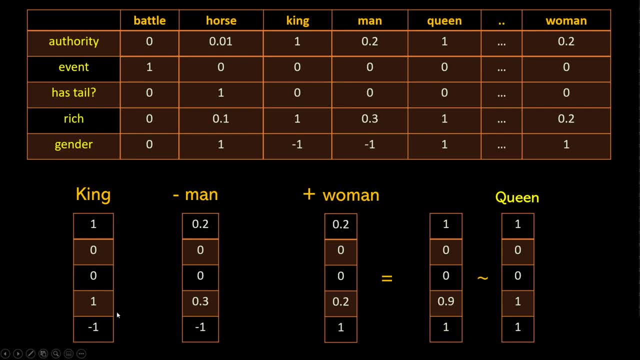 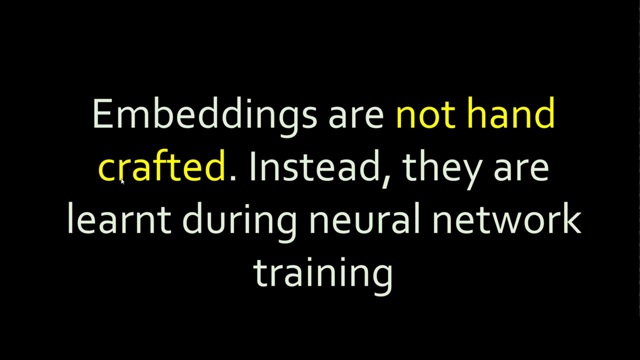 in computer programming you can use basically neural networks, uh, to learn these feature vectors. so these, these numbers are called feature vectors. okay, so authority event has still are called features in the language of machine learning. and using neural networks you can learn these feature vectors. you don't have to hand code it. so let's see how that is done. and, by the way, when you learn, 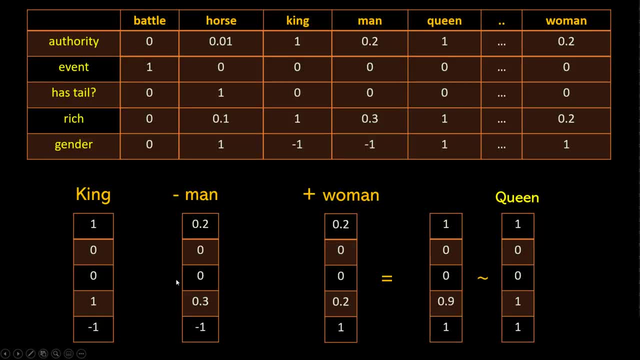 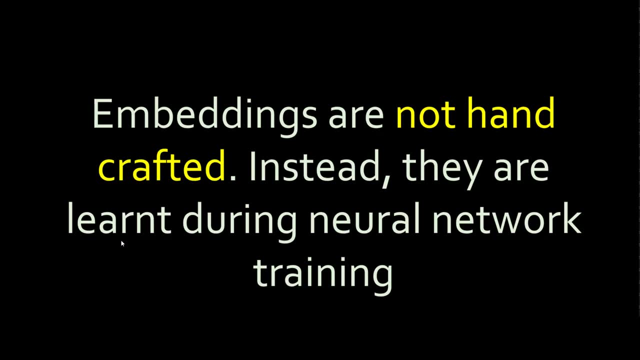 these feature vectors. one interesting thing about this is that when you add these features, you can thing that will happen is you will not know what these feature vectors are, You will not know that this one means authority, but it will all work magically. So what you do is you take a fake. 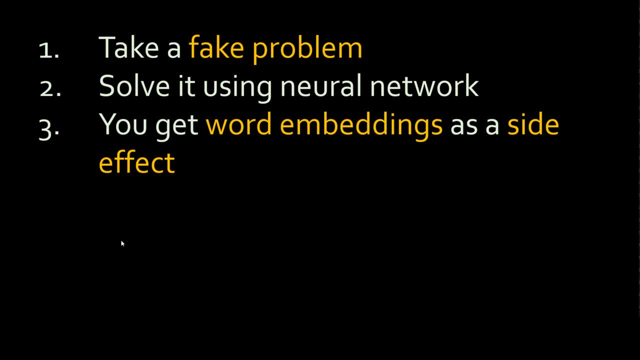 problem and you try to solve it using neural network And as a side effect, you get word embedding. Now what does that mean? So what is a fake problem? Let's say the fake problem is you want to find a missing word in a sentence. That's your fake problem. Well, the problem is real. but 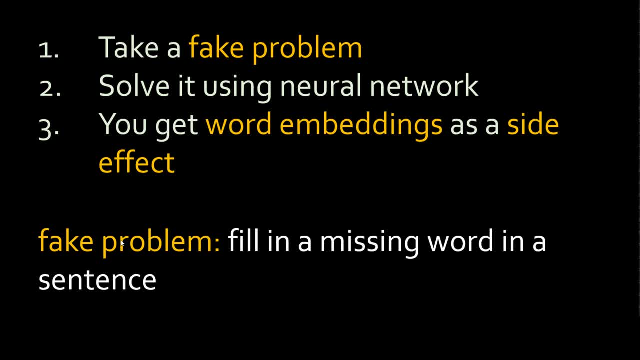 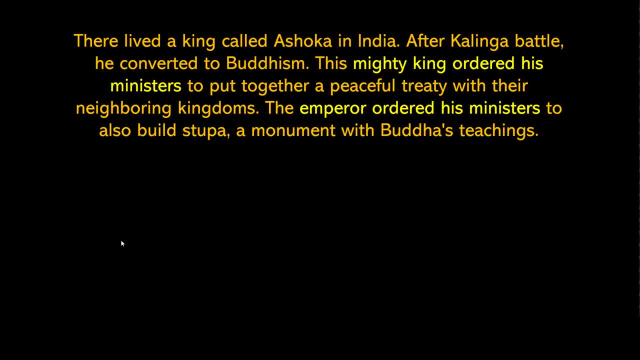 our goal is not to learn what is the missing word in a sentence. Our goal is to learn word embedding as a side effect. Say, there is a story of great king Ashoka. You know he was the king in India in ancient times And when you're reading the story you can take a fake. 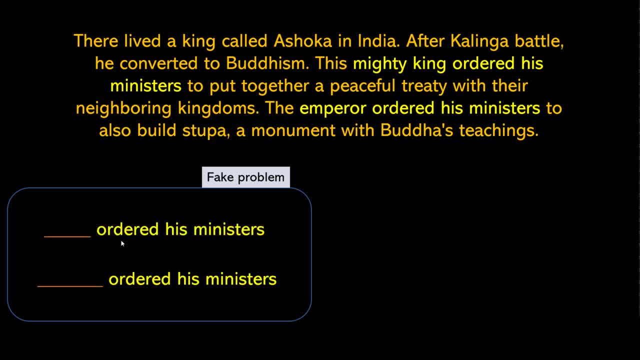 problem and you try to solve it using neural network And as a side effect, you get word embedding. So what you do is you take a fake problem which is complete. this sentence So here, when I say: order his minister. see, based on this text, this mighty king, order his minister. 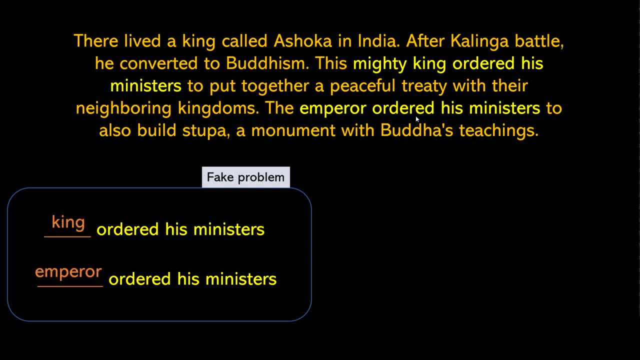 the emperor order his minister. I can say: the missing word is king or emperor. And when I give this task of filling in the missing word to a computer as a side effect, this is a very important keyword side effect. As a side effect, it will learn. 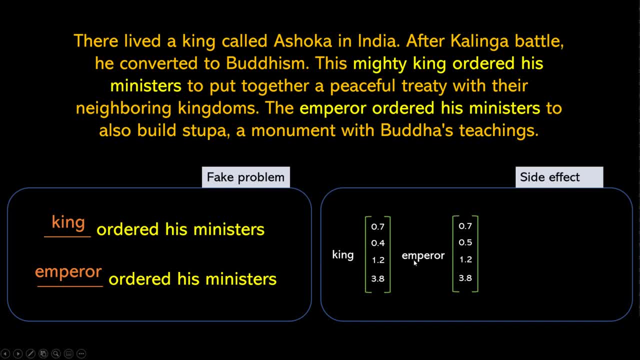 the vectors for king and emperor. These are those feature vectors. And once you have vectors, you can do math. You can say: king is almost equal to emperor. So see, you will be able to derive the synonyms, the antonyms. You can do math, such as: king minus man plus woman is equal to queen. 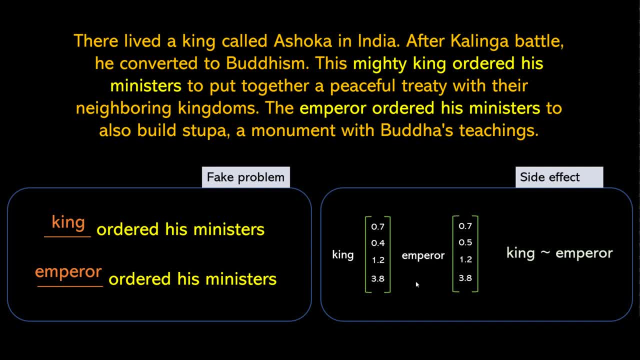 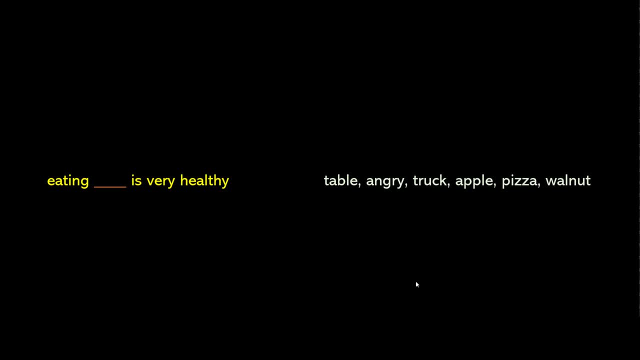 and so on. So now let's look into this problem a little further. For example, you have this sentence eating something, And if I ask you to fill in the missing word, well, most likely you will say apple and walnut, because that's food and that's healthy. Pizza is also food, but it's not healthy, So you won't. 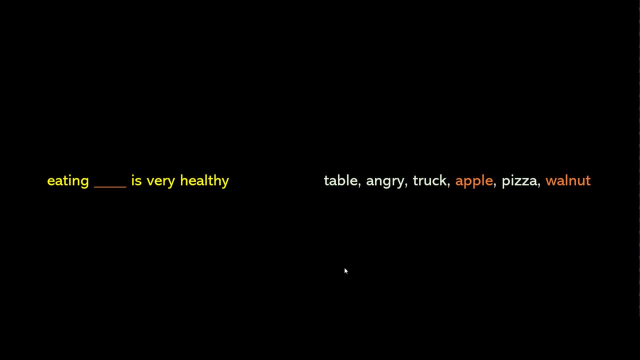 fill it and forget truck Eating truck is very healthy, Are you crazy? Similarly, when you have the sentence, the likely keyword will be rocket. You are not going to say: NASA launched pizza last month. so now, when you are in this process of finding out the missing word, you realize one fact which 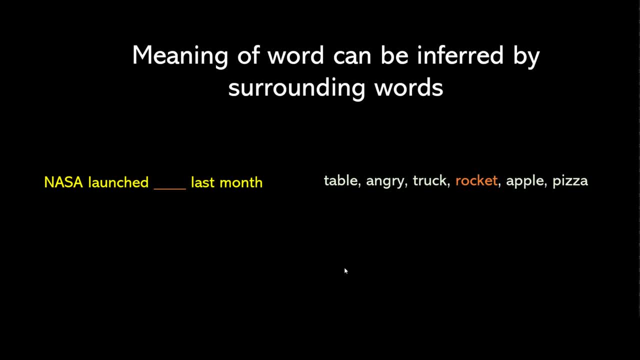 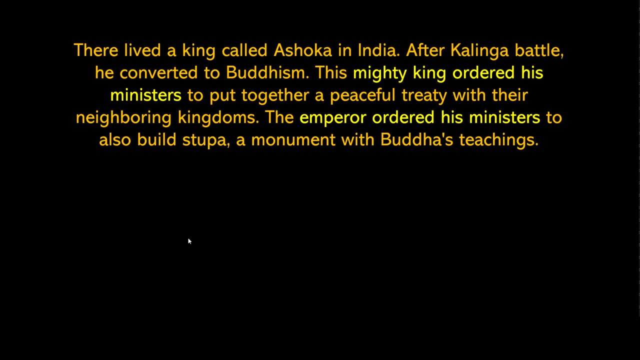 is meaning of a word can be inferred by surrounding words. if someone gives you surrounding words, so these surrounding words are also called context. so based on the context, you can figure out what that missing word is. so now let's take this paragraph and we will try to autocomplete those. 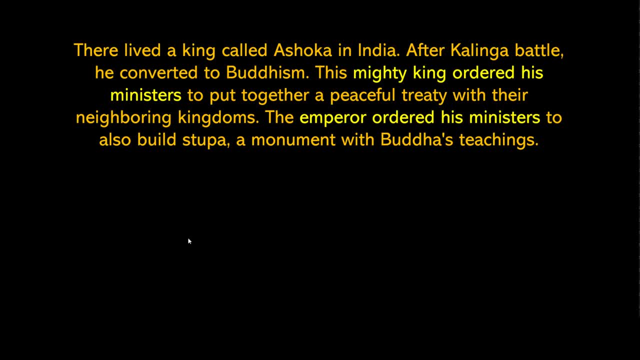 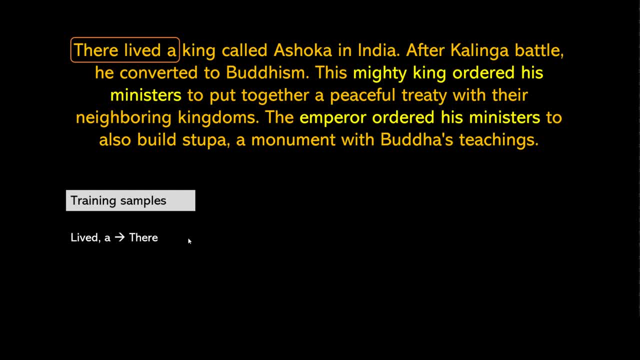 window of three words. and here i will say: if i have a word lived and a, i can predict that there is a word there. so i'm taking the second and third word and trying to predict the first word, and these are my training samples so i can move that window of three words throughout the paragraph. 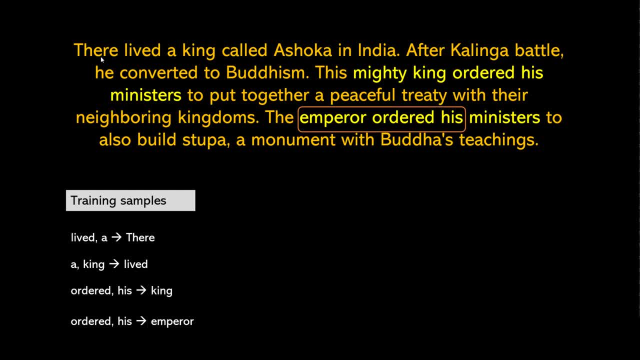 generate all these training samples. you see, i generated all these training samples and now this becomes a training set for neural network. so the words on the left hand side are my x, the word on the right hand side are my y, and you feed x into neural network and you want it to predict the word y. 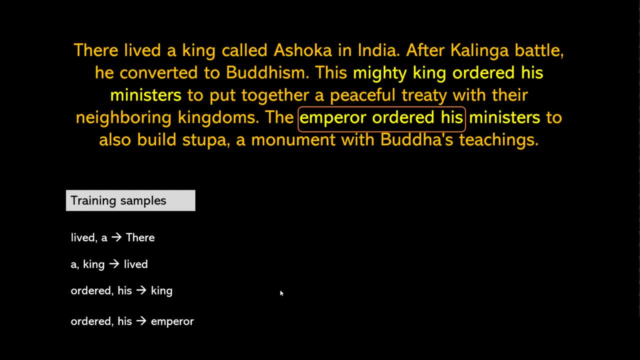 now. if you have not seen my neural network video, please go watch it. you need to have some understanding of neural network in under in order to understand things which i am going to explain in this video. so if you don't know already what is neural network pause? 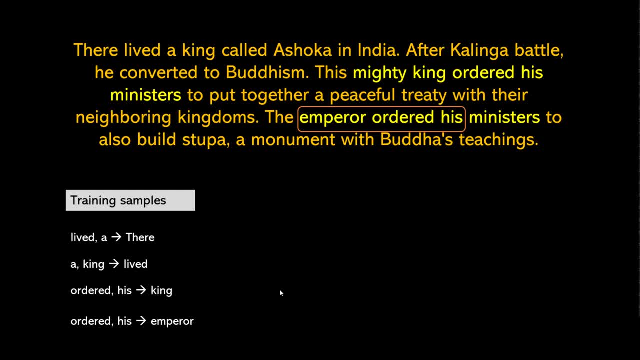 the video. right now i'm going to provide my neural network video link in a video description below. so just get some basic understanding, assuming you have the basic understanding. now let's go back to our problem, which is you have training samples and, by the way, this problem is called. 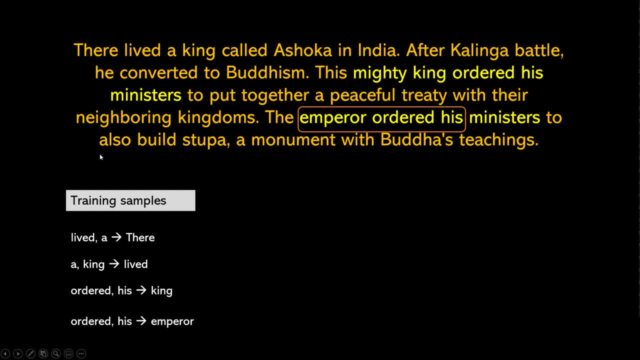 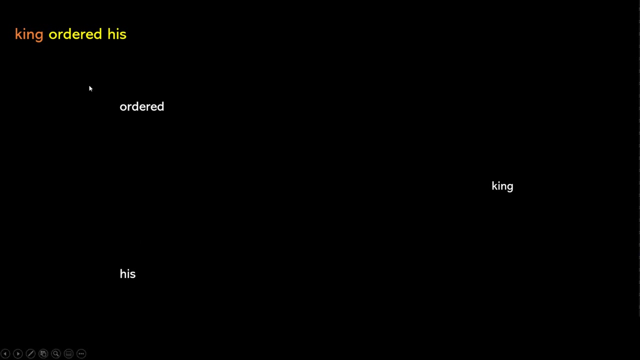 self-supervised, because all you had was this paragraph. you did not have like x and y, you had a paragraph. from that paragraph you generated these training samples. now let's try to train our neural network using each of these training samples. so let's have. my first sample is order his. so order his is an input. based on that, you want to predict working, which is. 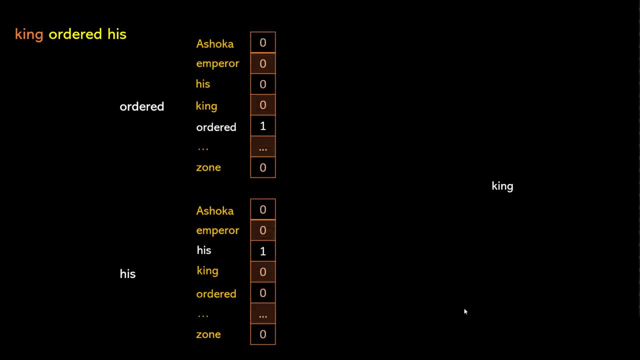 an output. now you can build a neural network that looks something like this: the input layer will have a one hot encoded vector. so let's say there are 5,000 words in my vocabulary, then there will be a vector of size 5,000 and only one of them will be one. so if the word is ordered, the value. 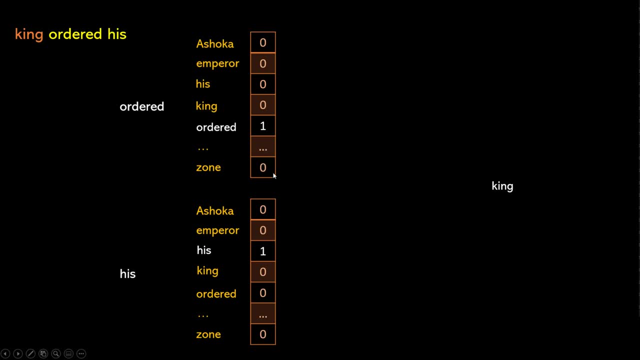 of order will be 1 and remaining numbers will be 0. and same thing is for his. see, his is 1 and remaining numbers are 0, and the size of this vector is, let's say, 5,000. 5,000 is, let's say: 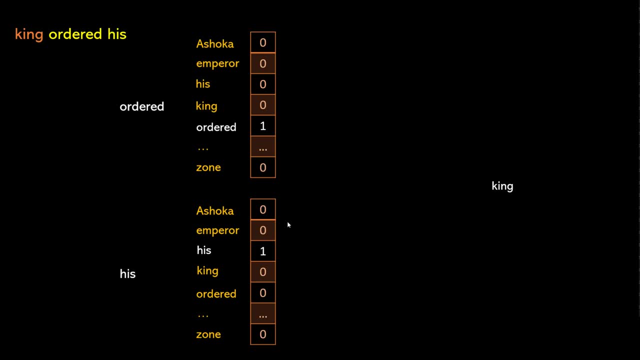 walk you. very vocabulary means unique words in your text corpus or in the you know text problem that you're trying to solve, and in the hidden layer here I have put four neurons and these four neurons are the size of my embedding vector. now, size of emitting vector could be anything like there is. 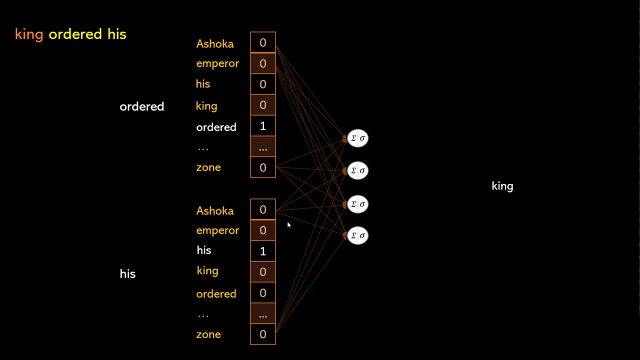 no golden rule. I just selected four, but it's a hyper parameter to your neural network. it could be five, ten, two hundred, anything. this is something you learn using trial and error. in the output layer, I will have 5,000 size vector and when I feed this training sample into my neural network, 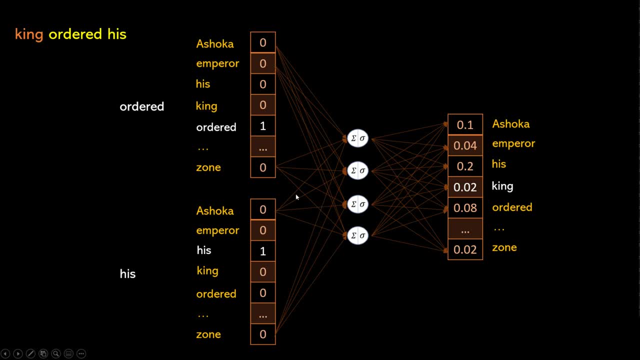 what happens is these weights, or the ages will have random weights. so using random weights, it will predict some output which will be wrong. most likely, King is the random most likely for NK. what does it predict? is that it will predict some output which is wrong. most likely, King is the383, and so on. 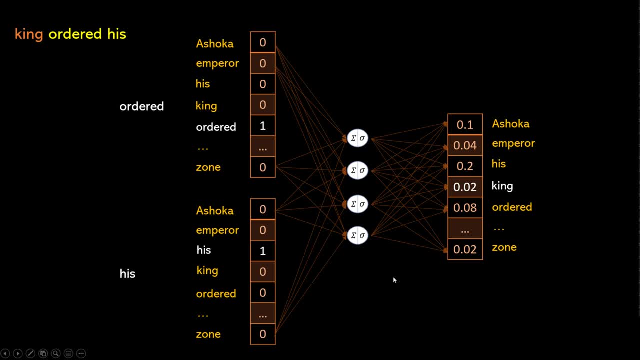 right output. so you all know how neural network works, how back error propagation works. you compare your actual output, which is y, with your predicted output, y hat. you take a loss. so loss is a difference between your predicted output and actual output, and you back propagate again. if you don't know, 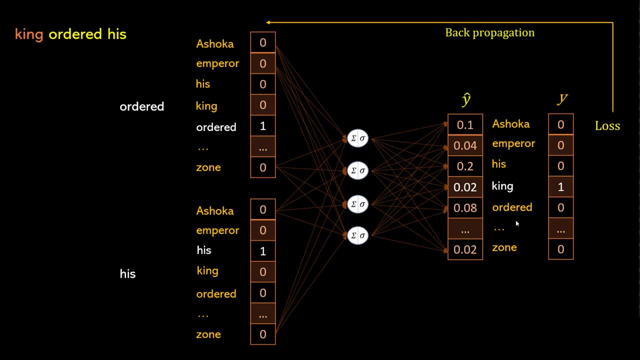 about back propagation. i have some videos, you can check it out. but when you back propagate, essentially what you're doing is you are adjusting all these weights and then you take us, and then you take a second sample, third sample. you take all ten thousand or one million samples and your goal 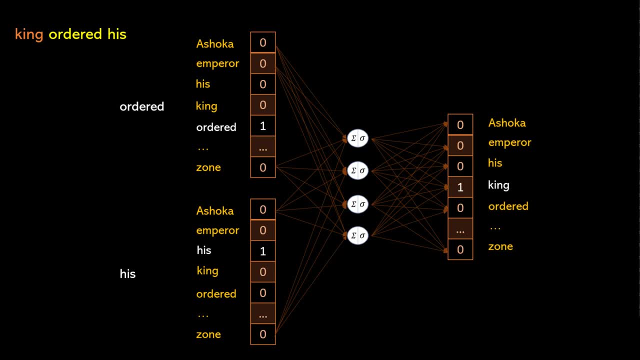 is to train a network in such a way that when you input order is the network accurately finds out that it is a king. so you expect one to be here. actually, you expect in the emperor here also. you expect it to be one because it could be anything. 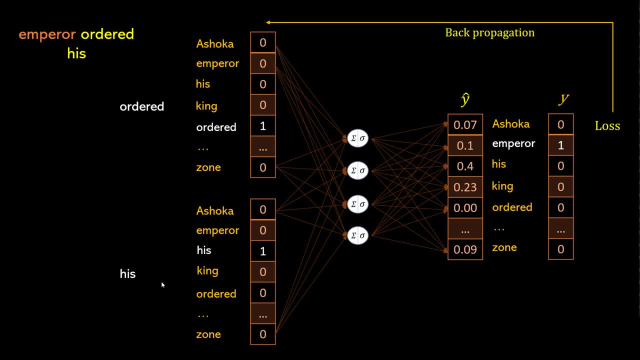 Now you take the second sentence, which is Emperor ordered his, and you're not taking the whole sentence. you're taking a window of size three. it could be window of size four or five, depends on you how you want to experiment. but same thing happens here: where you feed an input, the neural network will find out. 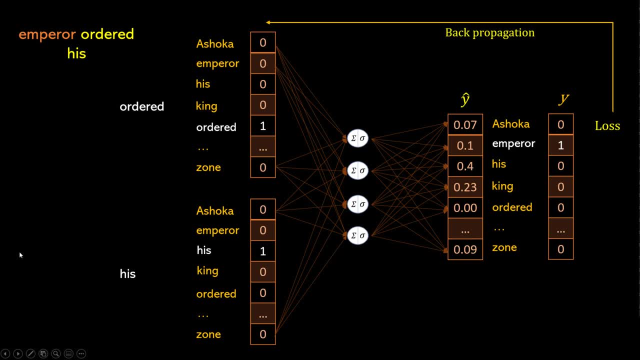 the output. it will compare it with the actual output. there is a loss and it will back propagate. and it takes the third sentence you know from Kalinga and battle. you're trying to predict that the missing word is after same thing. there is predicted output, actual output loss, back propagation and eventually, when you 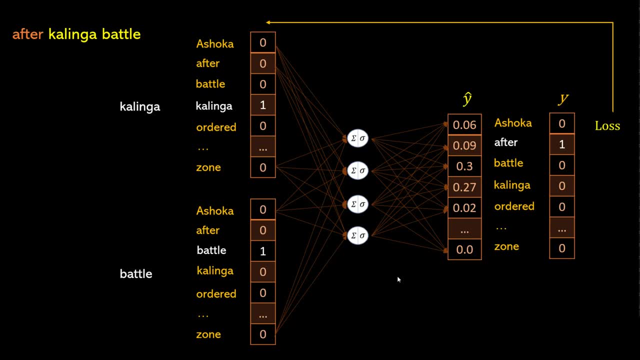 have done, you are done feeding your, let's say, 1 million elements and let's say you run 10 or 15 or 50 epochs and your neural network is trained. at that point, what is a vector for king would be these rates: w1, w2, w3, w4. so those weights are: 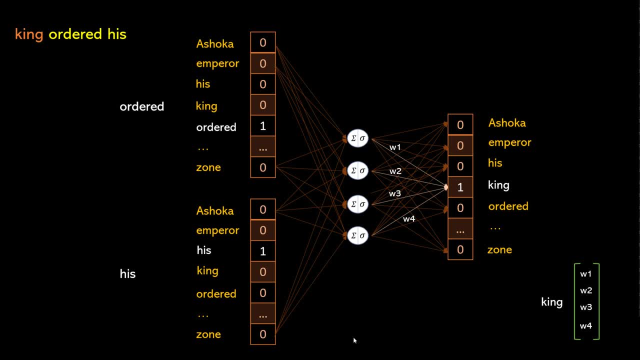 nothing but a trained word vector, and this vector will be very similar to a vector of Emperor. so the vector for the Emperor will be W 5, W 6, W 7, W 8. just think about it. it will be similar because the input is same. so here order. 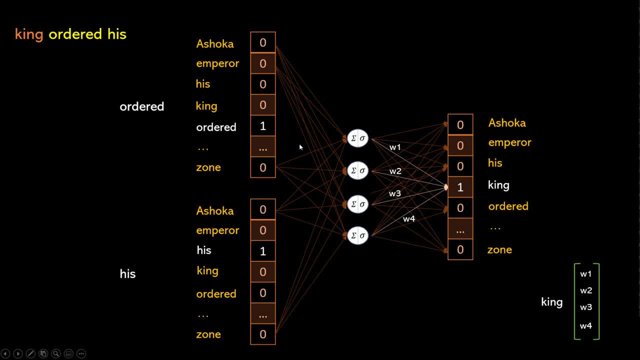 and his, both for King and Emperor and for the Emperor, and both for King and Emperor and emperor. the input is same. So when the input is same, you expect that these weights will also be similar, and hence the vector for king and emperor will be very similar. using this approach, 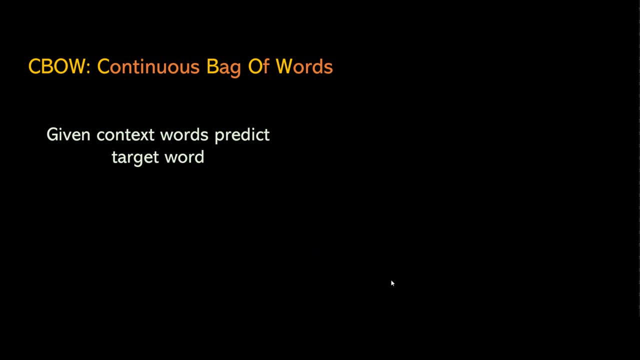 This approach is called continuous bag of words. So here you have a context which is order, his, and based on that context you are trying to predict target, which is king. There is a second methodology called skipgram. In skipgram we do reverse. We have a target word, king. 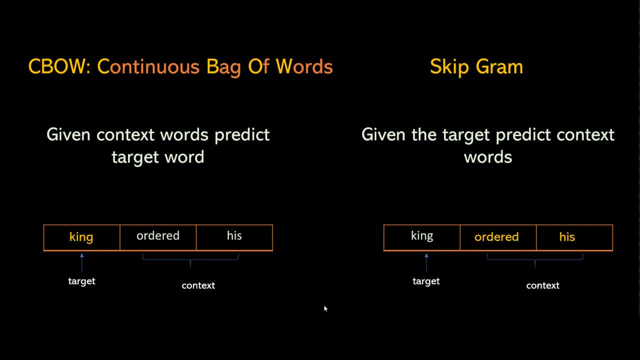 and based on that we try to predict order. his again, Predicting target from context and context from target. these are fake problems. You know we are not interested in solving this problem. But while we are trying to predict, solve those problems, as a side effect we get word embedding. so we are more. 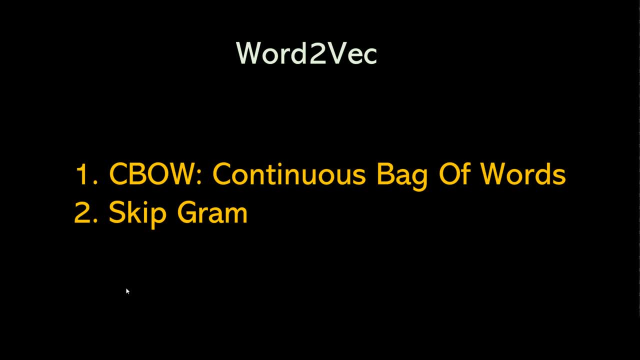 interested in learning word embeddings. just to summarize, word2vec is not a single method, but it it could be using one of the two techniques, which is either continuous bag of words or skip gram, to learn word embeddings: see the word. word2vec means convert word to a vector. so word2vec is a revolutionary. 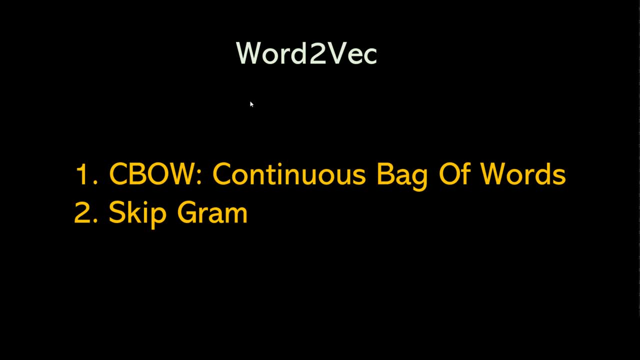 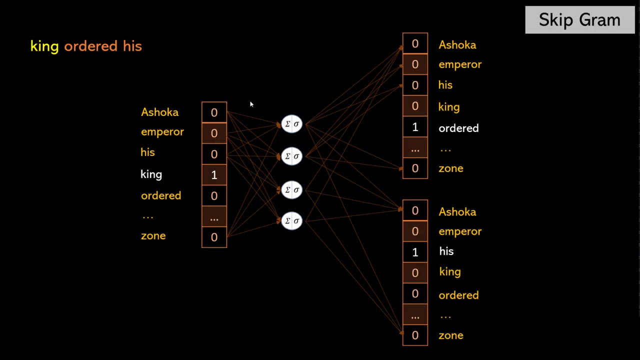 invention in the field of computer science which allows you to represent words in an, in a vector, in a very accurate way so that you can do mathematics with it. let's talk about script gram. since skip gram, I have inverted my neural network diagram, so here you can see: it's exactly reverse. 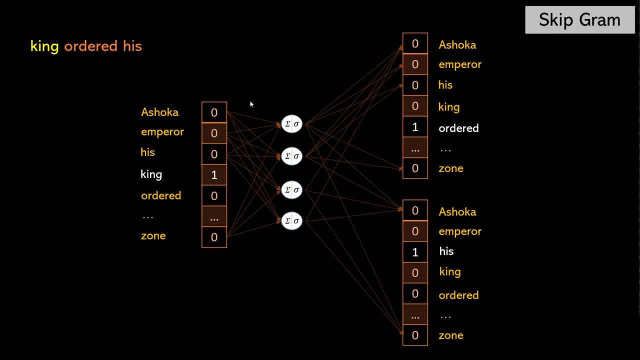 than the C bar. here you have the word King. based on that, you're trying to predict order, his, and you will do the same thing. you will feed one sentence, calculate the expected output, compare it with actual output, do back propagation and so on, and in that process you learn the word embeddings for each of these words. you know there. 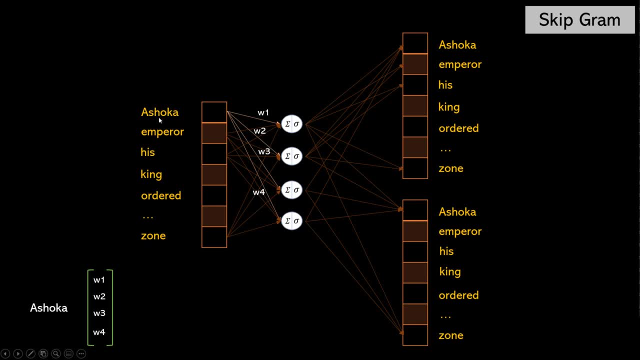 are 5,000 words less in our vocabulary. so the embedding for a Ashoka will be W1 to W 4. the embedding would be for emperor would be W6 to W9. so when you're using Skip gram, the word embedding is a layer between the input layer and the hidden layer in the C bar. it was 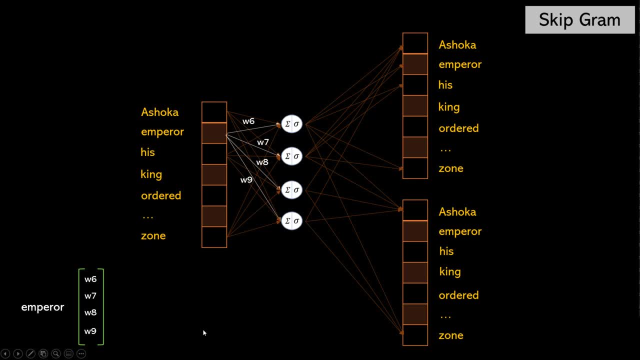 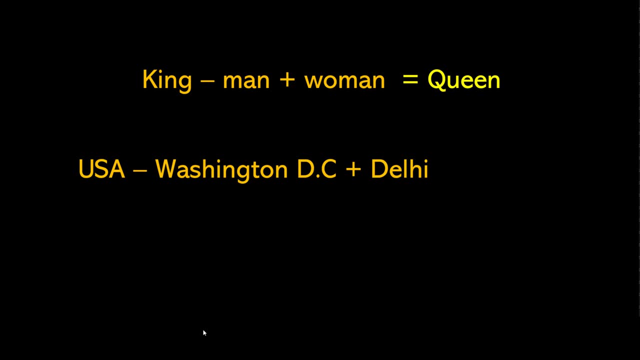 the weights between hidden layer and the output layer. You can do wonderful things with word2vec, such as USA minus Washington DC plus Delhi. Do you have any guess? pause the video. This is a quiz for you. Well, it is India. Okay, any guess on this one? 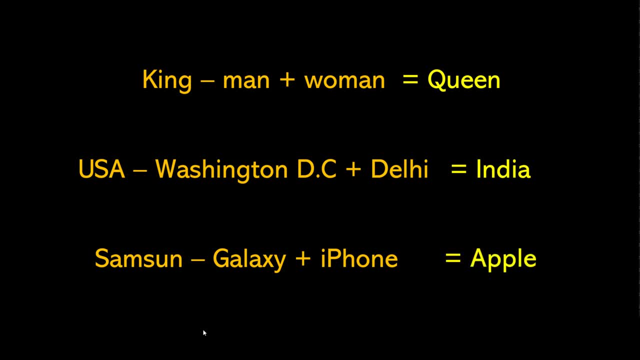 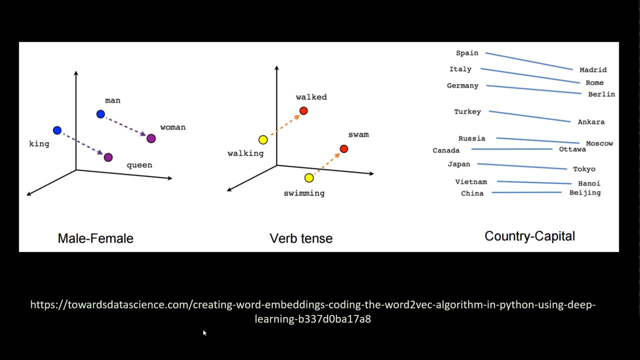 Wow, you all are so smart. Yes, Apple, so computers can do this kind of mathematics. This works really well. I Took this diagram from this to our science article. You can represent these Vectors in a vector space, So here I am showing you. 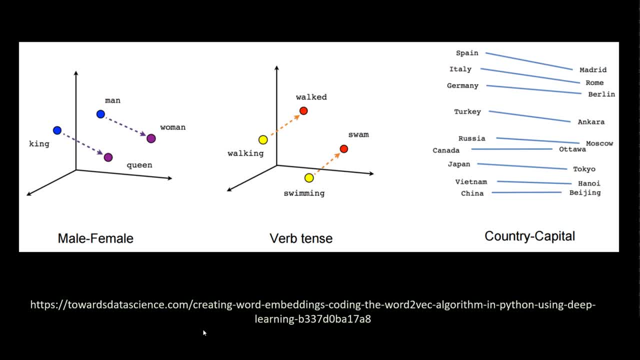 3-dimensional vector space. that could be n dimensional vector space and, you know, using a method called Disney, you can Chain that n dimensional vector space to two dimensional vector space and you will find that The word, The relationship between walking and walk will be similar to swimming and swam. 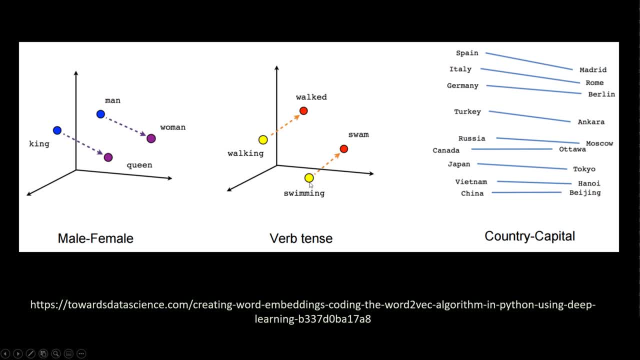 So once you have learned this relationship, when you give a word swimming to a computer, It will tell you the output is swam. It can also figure out a relationship Basically. it will say: okay, whatever is Madrid to Spain, the same thing is Rome to Italy. 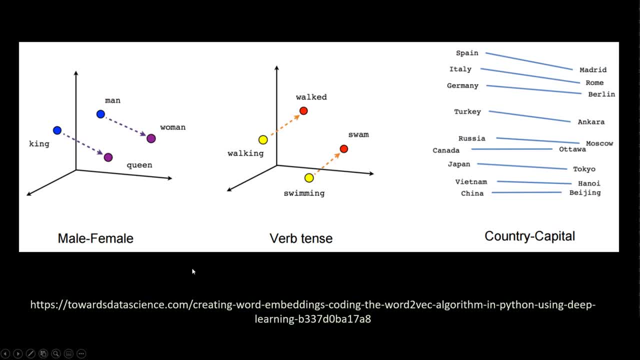 so it can run. it can learn these kind of Complex relationships. so that was all the theory behind Word2vec. I hope you liked this video. if you did, Please share it with your friends who are confused about word embeddings Word2vector, And if you have any question, post in a video comment box below. 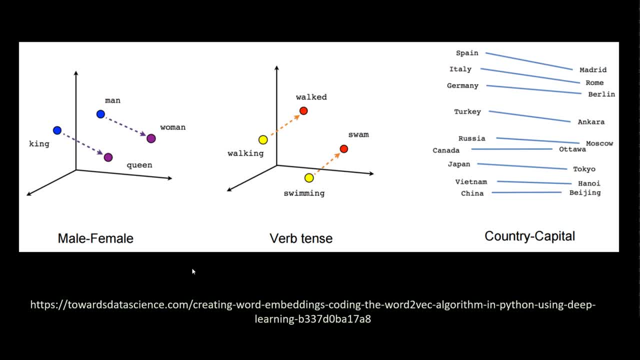 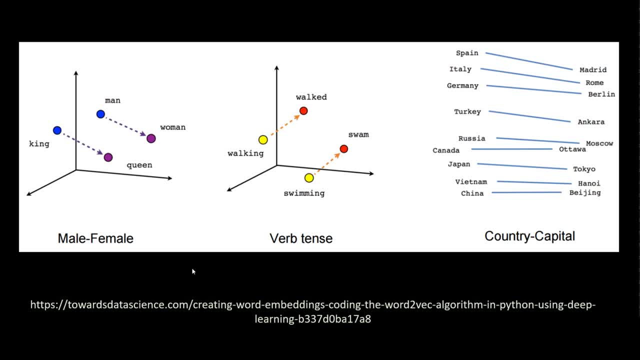 Python. we will see how word2vec works and will run some code or to see this magic in works. thank you,